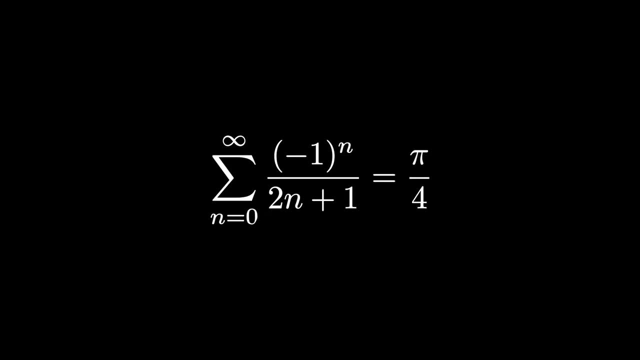 a very predictive test. When people think about math and formulas, they don't often think of it as a design process. I mean, maybe in the case of notation, it's easy to see that different choices are possible, But when it comes to the structure of the formulas themselves and how we use them, that's. 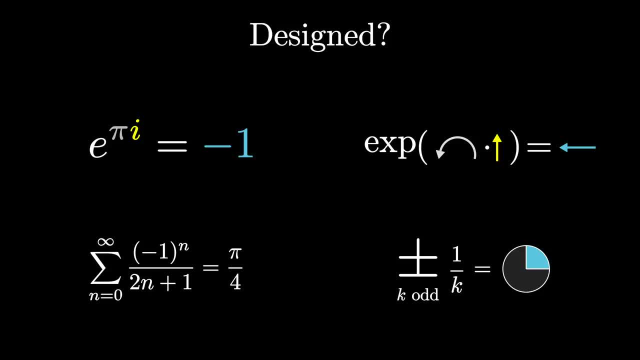 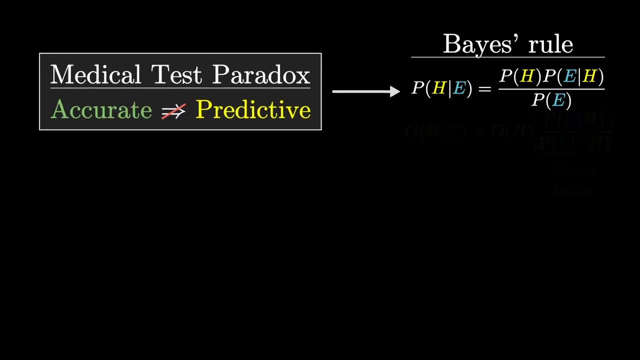 something that people typically view as fixed. In this video, you and I will dig into this paradox, but instead of using it to talk about the usual version of Bayes' rule, I'd like to motivate an alternate version, an alternate design choice. 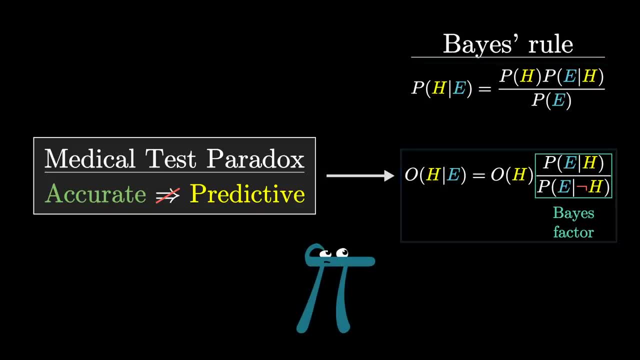 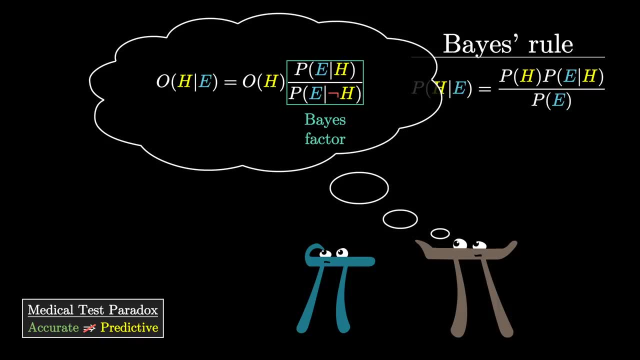 Now, what's up on the screen now is a little bit abstract, which makes it difficult to justify that there really is a substantive difference here, especially when I haven't explained either one yet. To see what I'm talking about, though, we should really start. 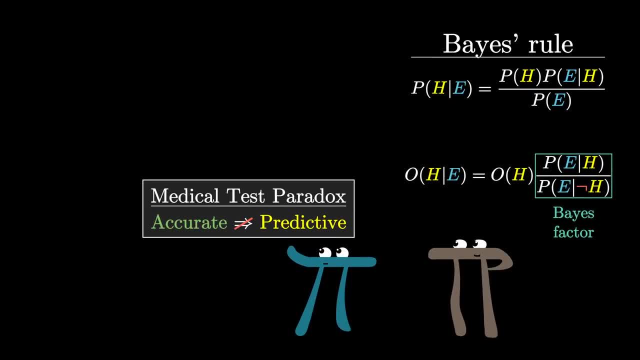 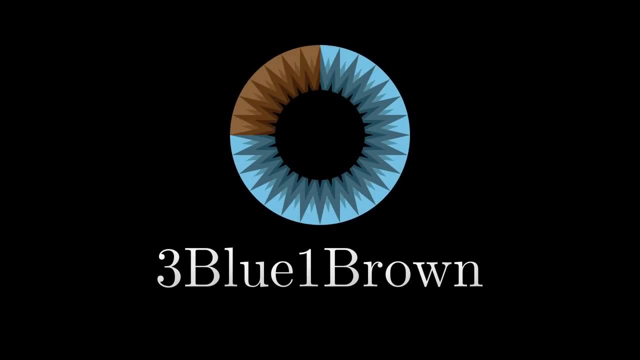 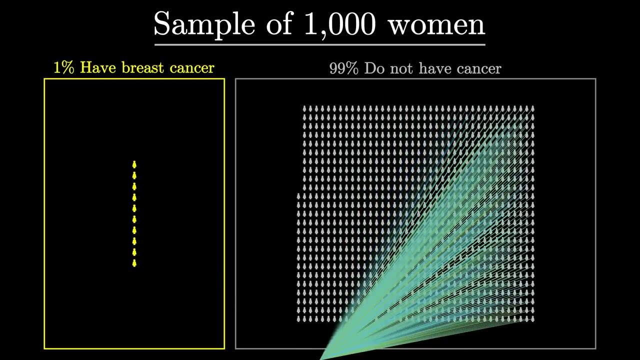 by spending some time a little more concretely and just laying out what exactly this paradox is. Picture 1,000 women and suppose that 1% of them have breast cancer And let's say they all undergo a certain breast cancer screening and that 9 of those with cancer correctly. 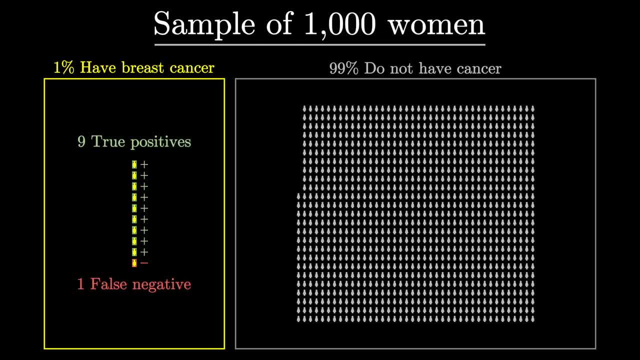 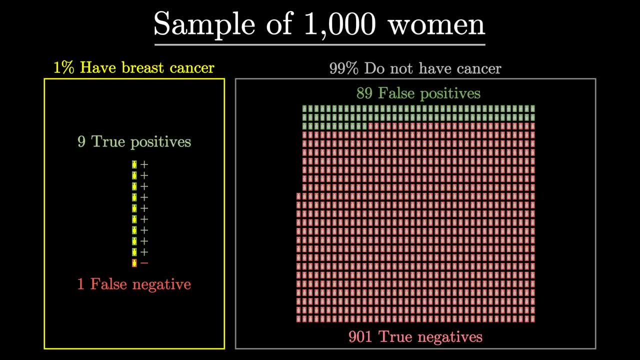 get positive results and there's one false negative. And then suppose that among the remainder without cancer, 89 get false positives and 901 correctly get negative results. So if all you know about a woman is that she does this screening and she gets a positive, 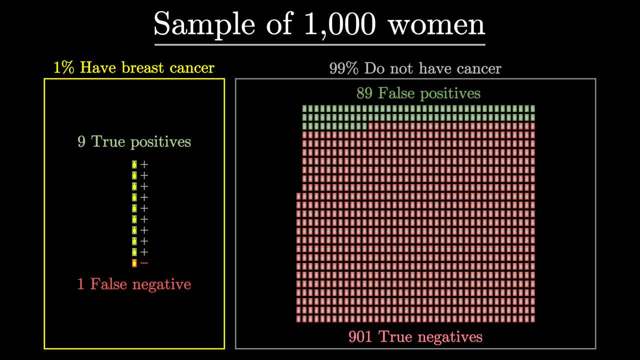 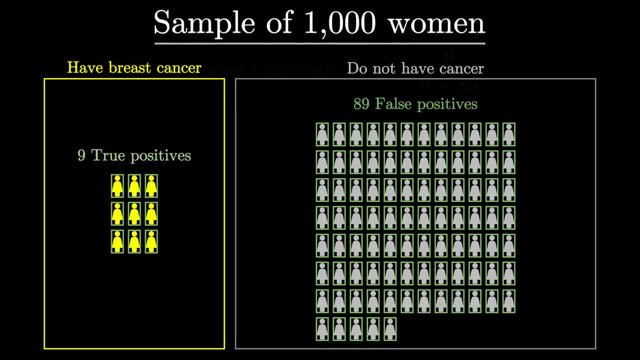 result. you don't have any information about symptoms or anything like that, then you're wrong. You know that she's either one of these 9 true positives or one of these 89 false positives. So the probability that she's in the cancer group, given the test result. 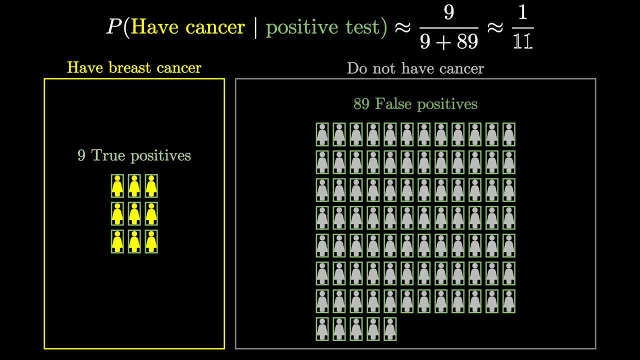 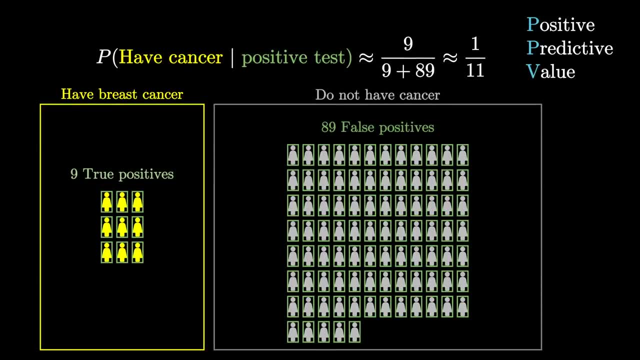 is 9 divided by 9 plus 89, which is approximately 1 in 11.. In medical parlance you would call this the positive predictive value of the test, or PPV, the number of true positives divided by the total number of positive test results. You can see where the name comes. 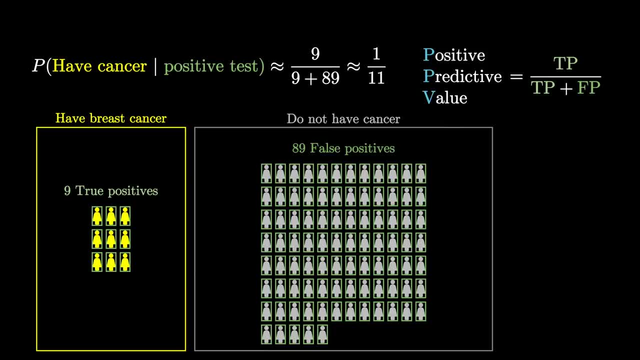